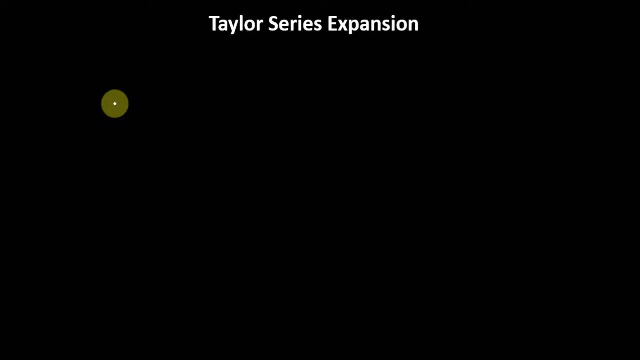 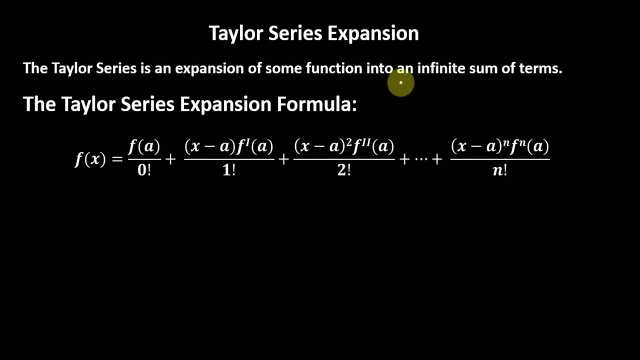 video as well. So let's get right into this video, guys. What is the Taylor series expansion? Now, the Taylor series is an expansion of some function into an infinite sum of terms. Now, based on the nature of the function, guys, the Taylor series can be used to find the cube root of a number and the square root of a number. 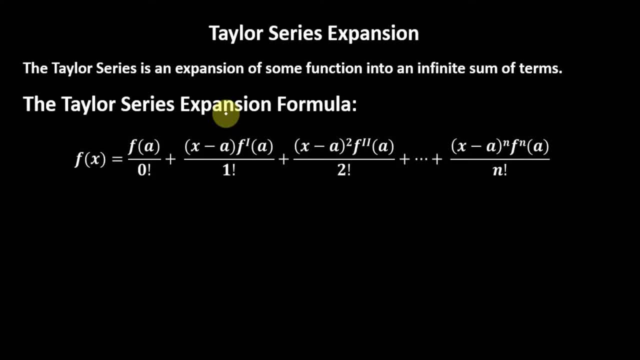 etc. So we can have an even, we can have Taylor series expansion for even trig functions, and I'll have an example of that in this video as well. Now the Taylor series expansion formula is: f of x is equal to f of a Over 0, factorial plus x, minus a in bracket times. the first differential of f of a. 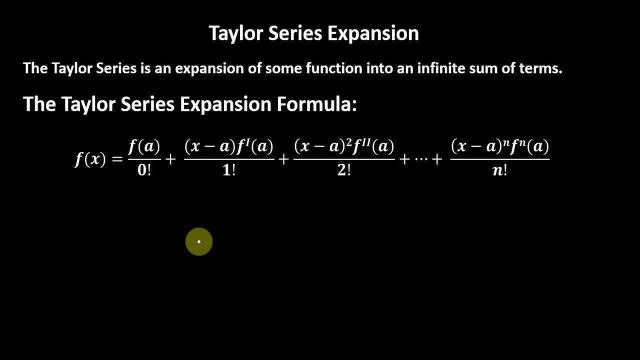 over 1 factorial, plus x minus a in bracket, raised to the second power times, the second differential of f of a over 2 factorial. And by now you get the sequence, guys, or the pattern for the Taylor series expansion formula. The next one would have been x minus a. 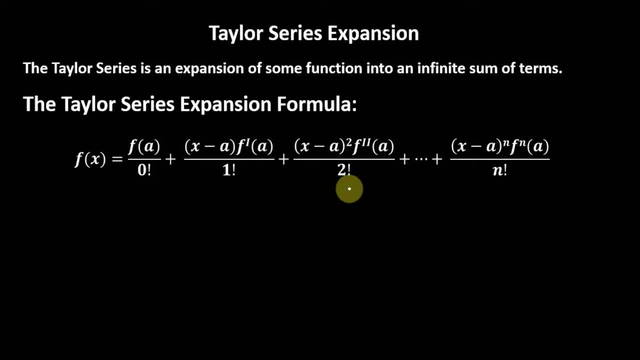 in bracket, raised to the third power times, the third derivative of f, of a over 3 factorial, And we can have an infinite sum of terms, guys. So that's why we have the three dots here to show that it continues. And the thing about the Taylor series, expansion, guys, the more term we have, the 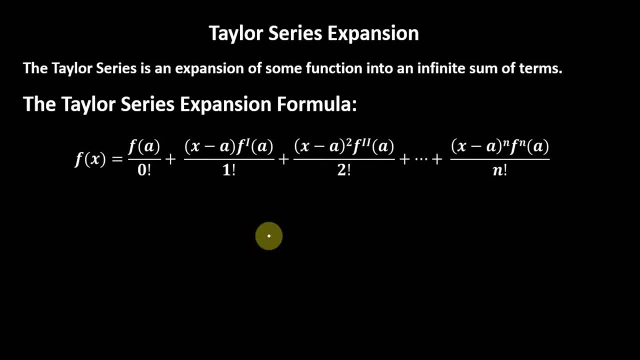 more accurate the series will be. Especially, let's say, we want to find the square root of a number. The more terms we have is, the more accurate the result will be, And you'll see that in our first example right here. So here we have question one. 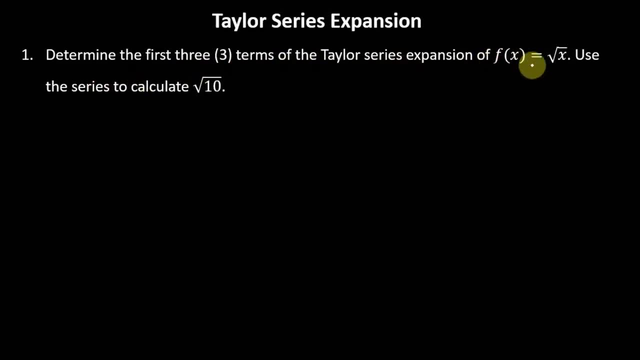 The first three terms of the Taylor series: expansion of f of x is equal to the square root of x, and use the series to calculate the square root of 10.. Now we have to bear in mind that we want to use a series to calculate the square root of 10.. 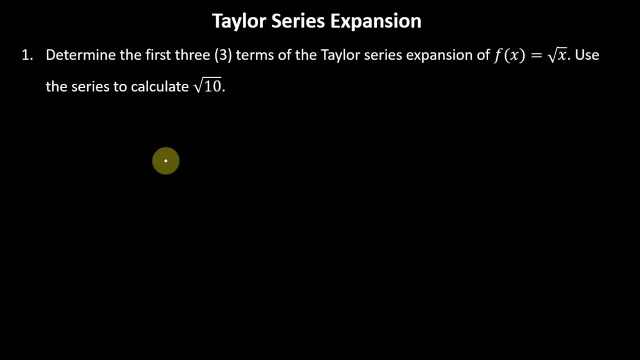 Now, the first thing that we want to look at, guys, is our function. By having the function here, we'll know what we need to find. in order to write the first three terms of the Taylor series, expansion for the function f of x is equal to the square root of x. bearing in mind that we want to 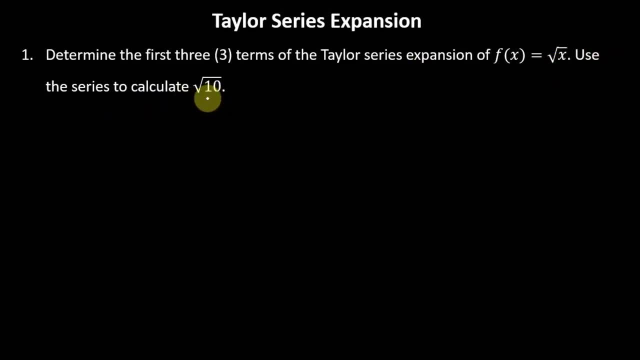 use a series to calculate the square root of 10, and you'll find out soon, guys. it's quite easy. nothing really, to it. so here we have the formula again, guys. now we're going to need our f of a, the first differential of f of a and the third differential of f of a. so these are the first. 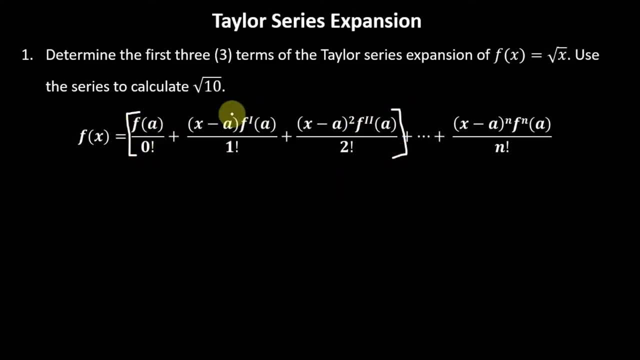 three terms right here. so we're going to need these values. now, the key thing here, guys, before we go on and differentiate, we're going to need a value for f of a, not just the function. so, um, the key thing here, guys, is to find out what is our a value, or how do we choose our a value if 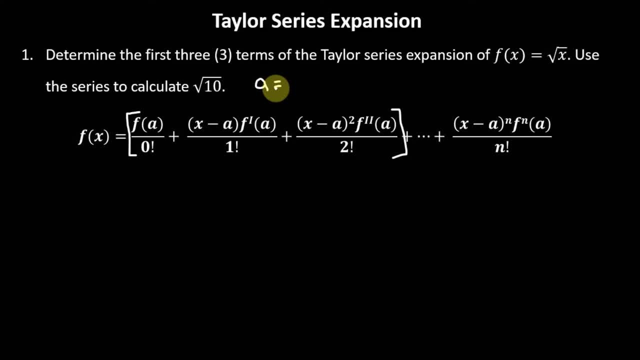 we're not given the a value in the problem now, bearing in mind, the a value is dependent on the function and what we want to use the series to calculate. now the function is f of x is equal to the square root of x. we want to use the series to calculate the square root of 10. now we want to find the. 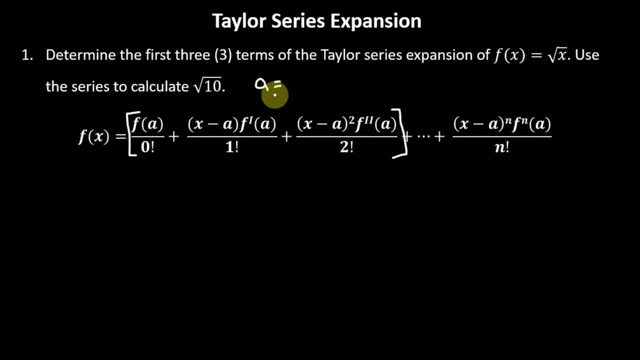 closest perfect square to 10? because 10 is not a perfect square, meaning that if we should square root 10, we'll not get a whole number for the answer, we'll get a decimal value. so we want to find the closest perfect square to 10. which number is the closest perfect square to 10? 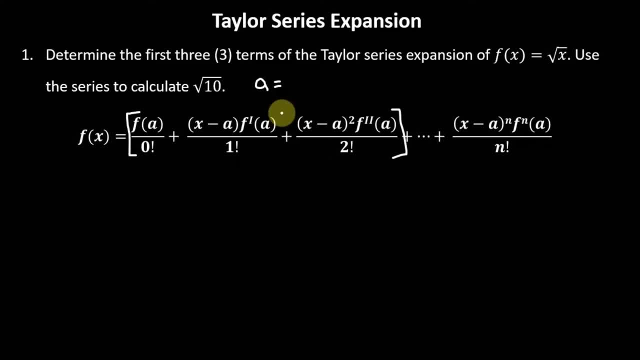 number is closest to 10 that we can find the square root of, and the result will be a whole number. there you go. that number will be nine and that is how we choose our a value. all right now, after choosing the a value, guys, we can go ahead. we are going to find f of a, and the first 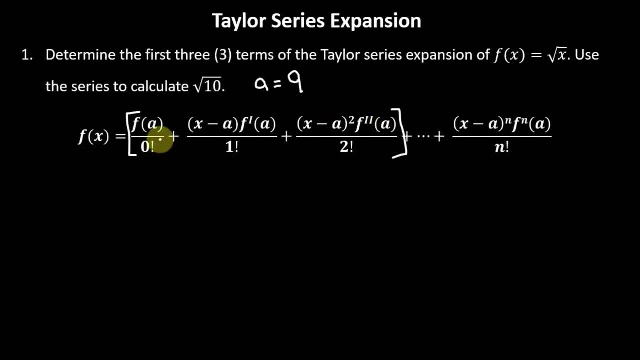 differential of f of a and the second differential of f of a, because we are going to need these values for our first three terms. all right, so we are going to go ahead and find our f of a and the second differential of f of a, so our f of a. bear in mind that f of x is equal to the square root of. 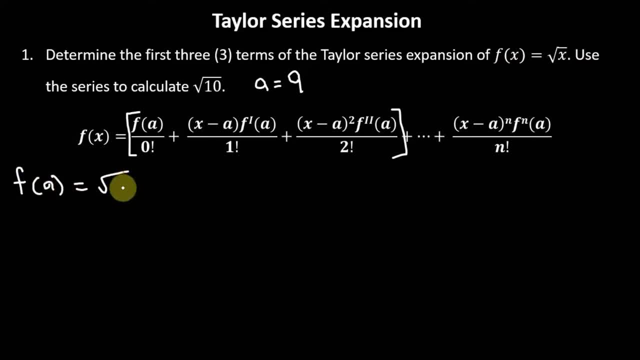 x. so therefore f of a will be equal to the square root of a. remember, guys, that way we have outlined that our a value is 9, so therefore we can say f of a is equal to the square root, or a value is 9, square root of 9. square root of 9 is, of course, 3, and that's pretty much how we find our f of a. 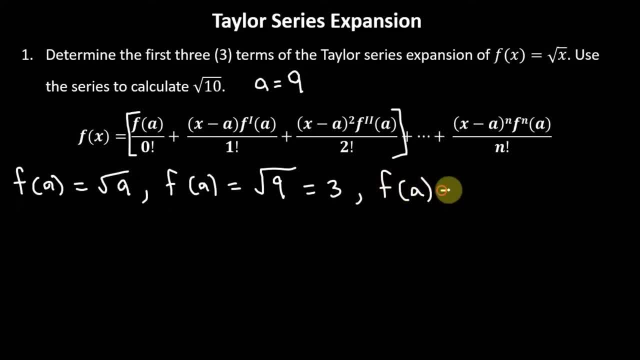 and this is our f of a 3. i'm going to have this value here, guys, because we're probably going to have to erase this section of the board to get some more space, so i'm going to write it up here. f of a is equal. 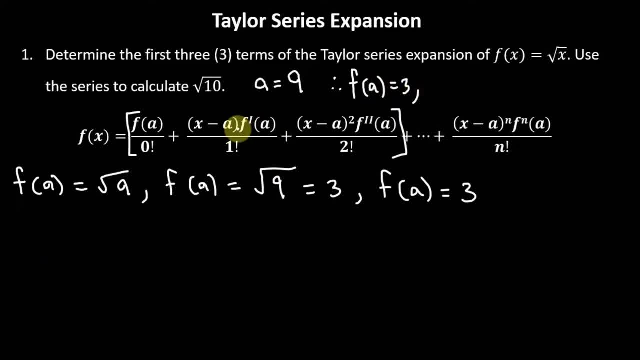 to 3. now i want to find the first differential of f of a, first differential of f of a, which means we are going to have to differentiate the f of a function. now bear in mind, guys, that the square root of a is the same thing as a raised to the power of a half. 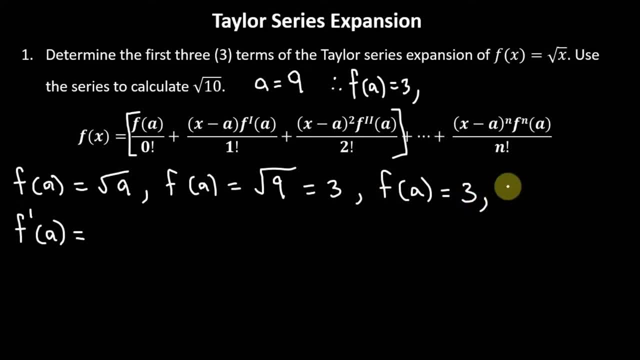 all right. so let me put that out here, just in case you're struggling to picture that in your mind. so f of a is equal to a raised to the power of a, half same thing as a, the square root of a. all right, so the reason why i write it like this, guys, because we are going to differentiate this. 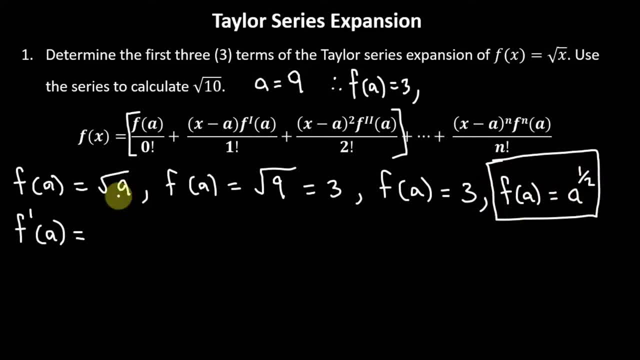 and it's probably easier to differentiate this than to look at the square root sign right here. so, um, being that we know that the square root of a is the same thing as a raised to the power of a half, we can differentiate the function, a raised to the power of a half. now, we're going to differentiate this using the power. 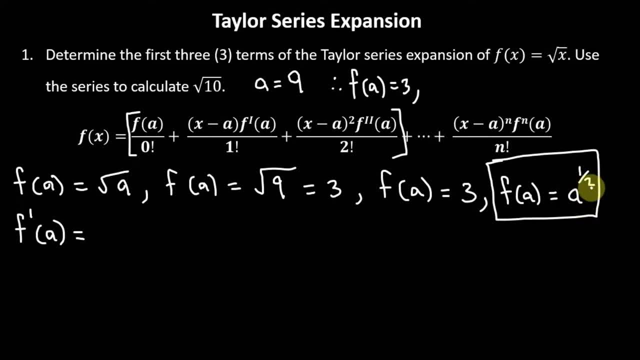 rule. so we are going to multiply by the power. then we're going to subtract one from the power. so in multiplying by the power we'll end up with what? a half times 3, and that's going to be the square root of a. so we're going to multiply by the power. 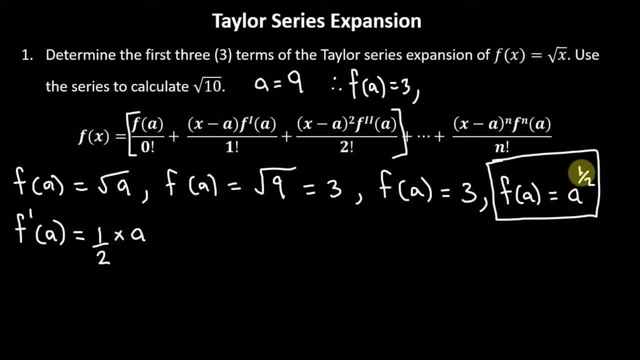 a, we'll subtract one from the power. a half minus one is, of course, negative one over two, and we can clean this up a little bit, guys. all right, you can clean this up. so we have: f of a is equal to, and this is the same thing, of course, one times. 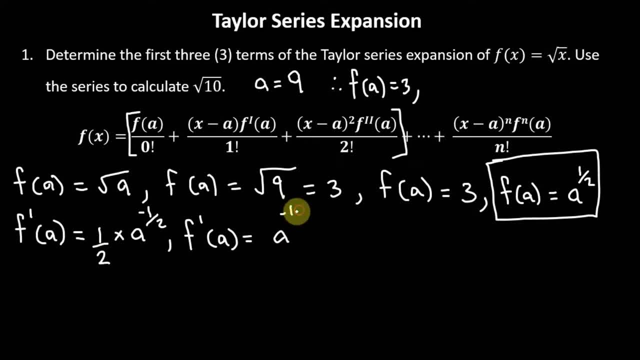 a raised to the power of negative a half is a raised to the power of negative a half, and we'll have the two in the denominator here. we can even go a step further and clean this up using the laws of indices here. so this is the same thing as one over two. 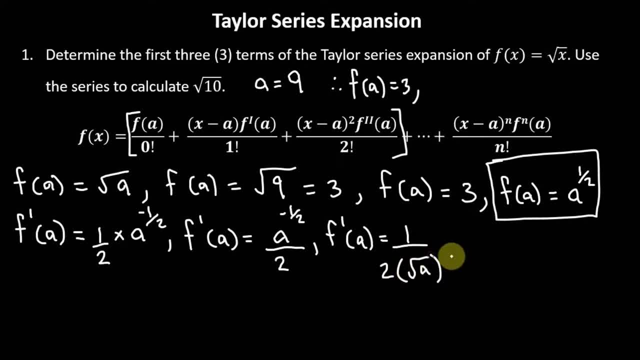 and in bracket we can have the square root of a. so we use the law of indices there to write it in a form so that we can plug in our a value and it's probably easier to use. all right, so we'll have one over two and in bracket we'll have the square root of nine and this will be. 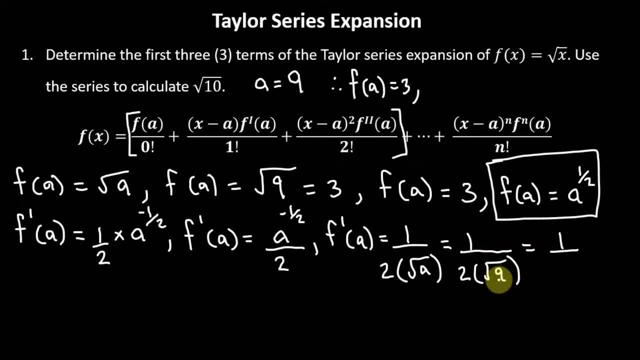 equal to one over. let's see: the square root of nine is of course three. two times three is six. so therefore the first differential of f of a is equal to one over six, and i'm going to write that here. so the first differential of f of a 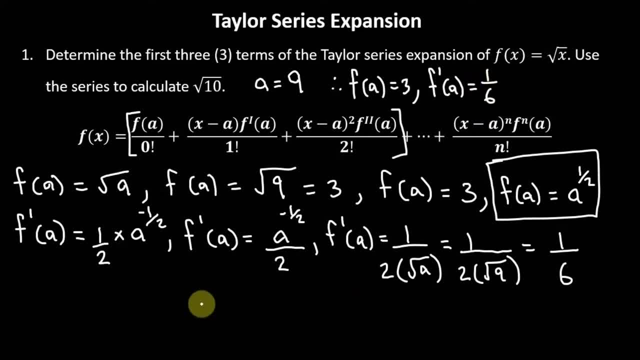 is equal to one over six. all right, and we are going to continue. so we need to find second differential of f of a and to do this we're going to need the, the first differential of f of a function, and we can use this one here. we're going to use this one, all right. so we're going to multiply by the power. 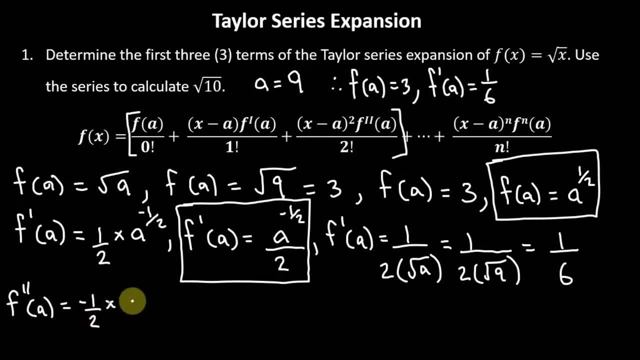 so we'll have negative one over two times. we have a raised to the power of negative a half here over two. remember, guys, we're going to take one from the power. if we take one from the pole, we'll have minus a half, minus one, which will give us 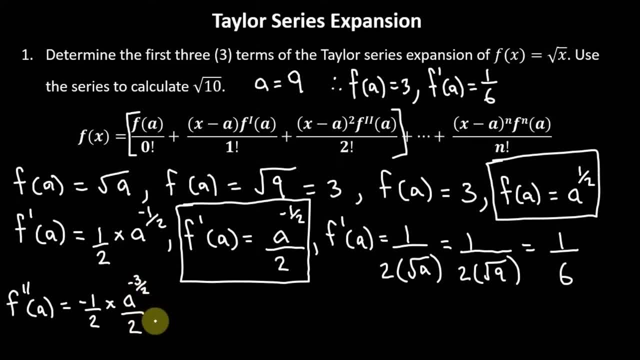 negative three over two. and of course, guys, we again we can clean this up a little bit so we have: second: differential of f of a is equal to. we can multiply this out so we'll have negative one times a is of course negative, a raised to the power of negative three over two. 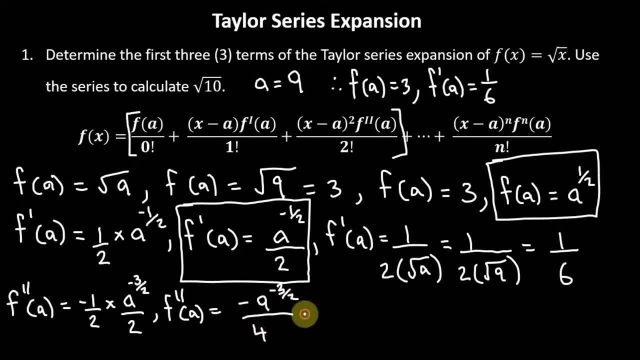 over two times two is four, and here we can go a step further, using again laws of indices to our benefit. so we'll have negative one over four and in brackets, here we'll have the square root of a in bracket cube. remember guys, our a value is nine, so we can replace. 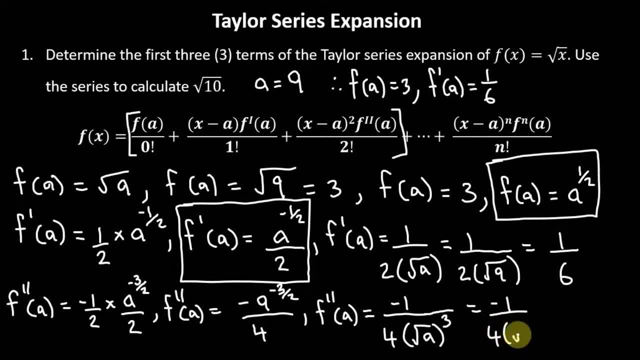 our a with nine. so we have four bracket square root of nine and we're going to cube it and let's see what this gives us. so we'll have negative one over the square root of 9 is, of course, 3,. 3 cubed is 27, and of course, 4 times 27 is 108.. 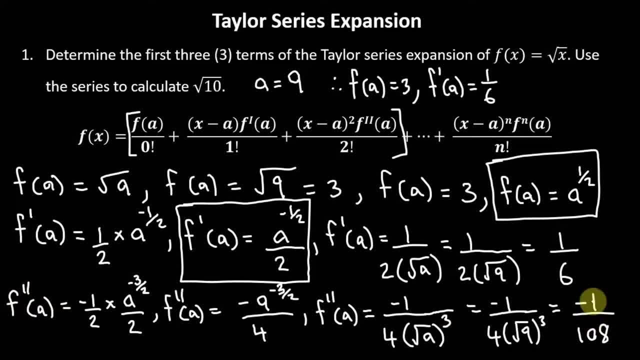 So therefore, the second differential of f of a will give us negative 1 over 108.. So the second differential of a is equal to negative 1 over 108.. And that is pretty much the majority of the work, guys. So I'm going to clear this space so we can write out the first three expansions. 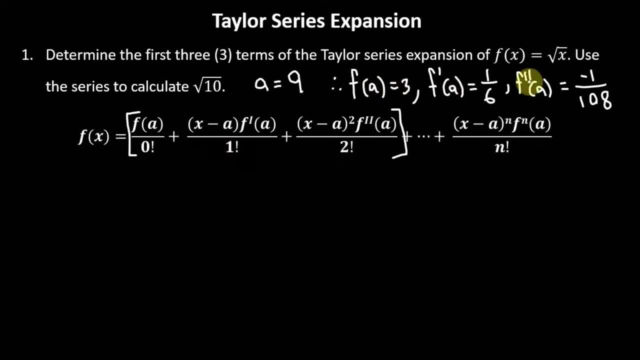 Now to write out the first three expansions. guys, we're going to need these three values that we just found And we're also going to follow the formula here. So we're going to have our: f of x is equal to f of a. 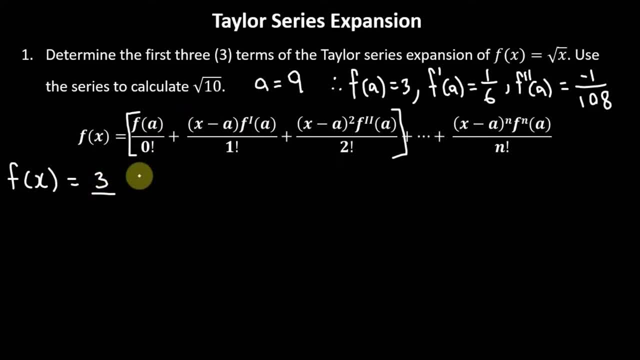 Of course, f of a. we found that to be 3 over 0 factorial, which is 1.. Plus, we're going to have the first differential of f of a times the bracket here, which is x, minus a Recall, guys, that our a value is 9, so we can replace a in the bracket here with 9, which is what we're going to do. 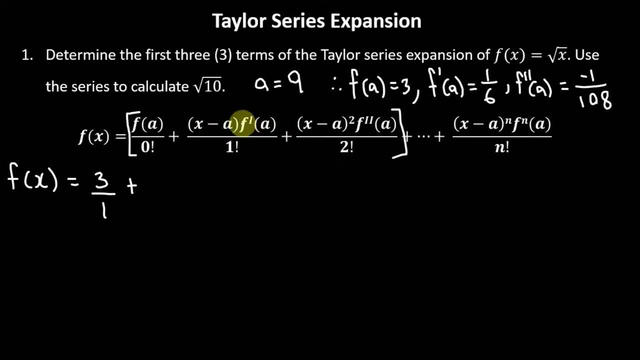 So it doesn't really matter. The order of multiplication doesn't really matter here. So we could have had the first differential of f of a at the front, which is how we are going to write it. So the first differential of f of a is 1. sixth, 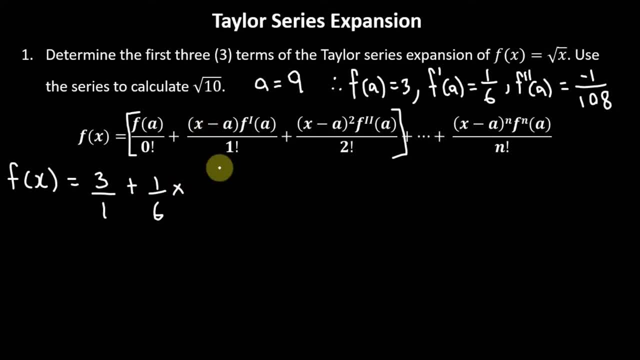 So we'll have 1 sixth times the bracket here, which is x minus a, And again our a value is 9 over 1 factorial, which is 1.. Plus, we're going to put the value for our second differential at the front again, just like we did the first differential value. 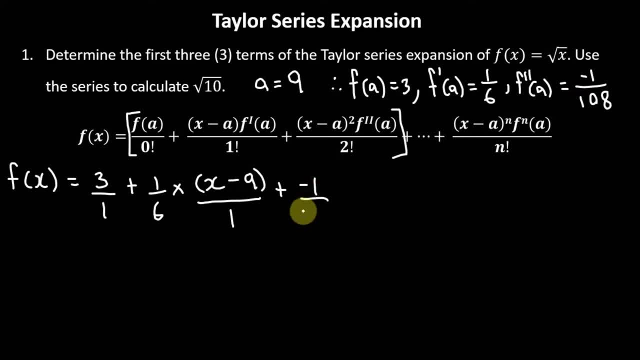 So we're going to put our negative 1 over 1 eighth at the front times. the bracket here x minus a, And again our a value is 9.. And we're going to raise this to the second power, just the same, over 2 factorial, which is of course 2.. 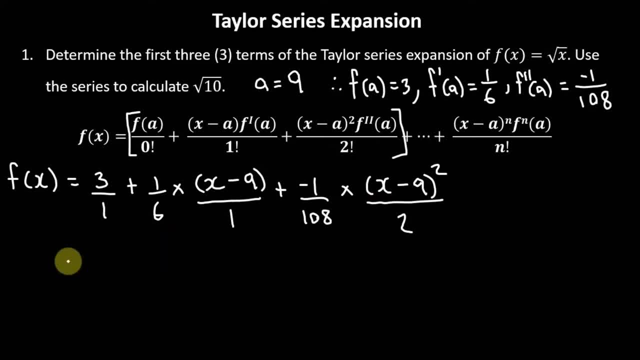 And these are the first three terms, guys, And all we need to do here is just to clean this up a little bit. So f of x is equal to 3. divided by 1 is, of course, 3, plus 1 times the bracket here. 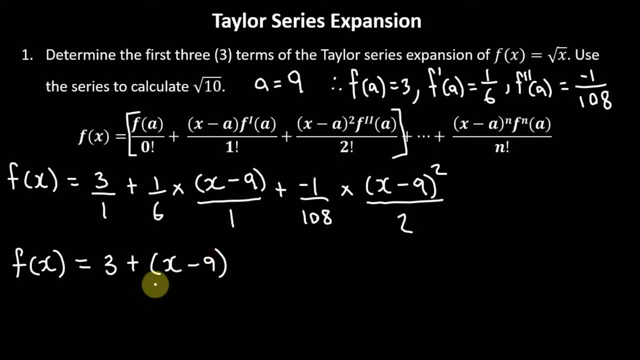 Bracket will remain x minus 9.. Over 6 times 1,, which is 6.. And whenever we have a positive and a negative sign like this, it's always equivalent to a negative sign. 1 times the bracket here raised to the power of 2, will remain x minus 9. in bracket raised to the second power. 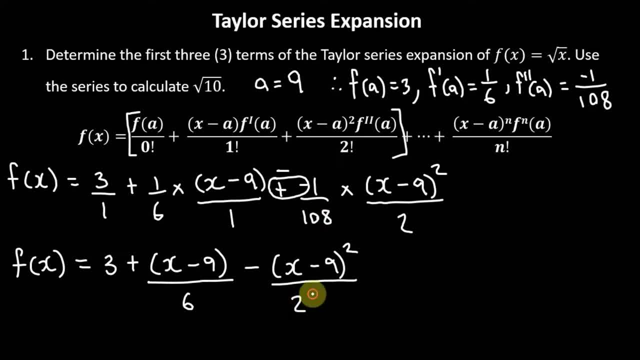 Over 108 times 2,, which is 216.. And these are the first three terms of the Taylor series expansion. So f of x is equal to the square root of x, And we'll bear in mind that we want to use a series to calculate the square root of 10, which is what we are going to do next. 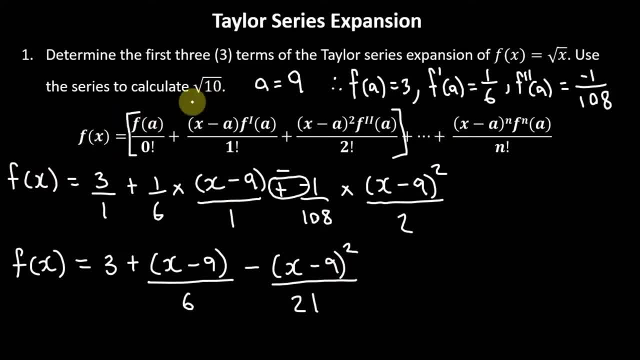 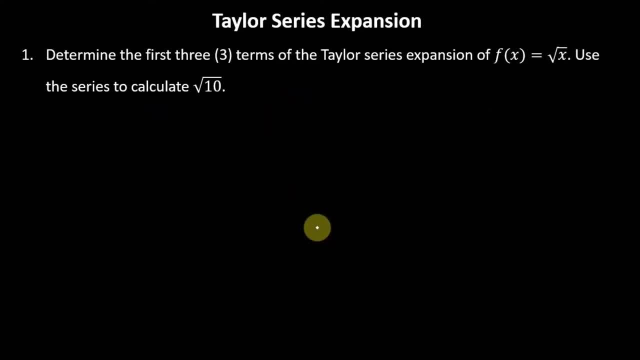 Now let us erase this space and use this series to calculate the square root of 10.. Now we want to use the series that we just found, guys, to calculate the square root of 10.. Now, recall the series. So there we go. 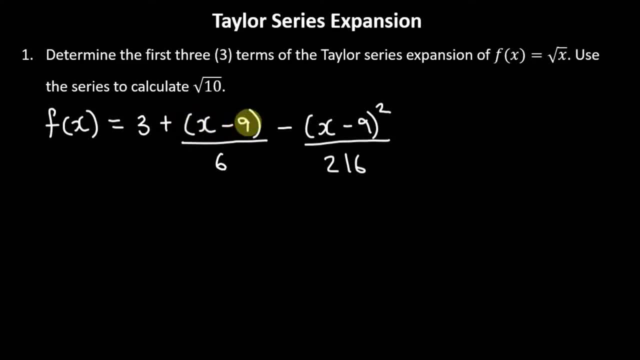 f of x is equal to 3 plus x minus 9 in bracket, all over 6, minus x minus 9 in bracket, squared over 216.. So we want to use this series to calculate the square root of 10.. 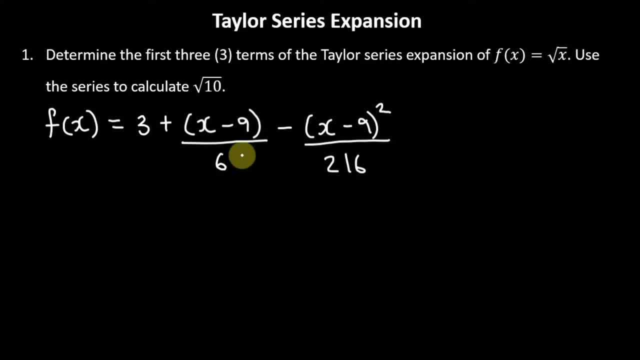 Remember, guys, that these first three terms they are Taylor series. expansion for the function f of x is equal to the square root of x And we use our a value with respect to the 10 right here. So they should give us a close value to that. 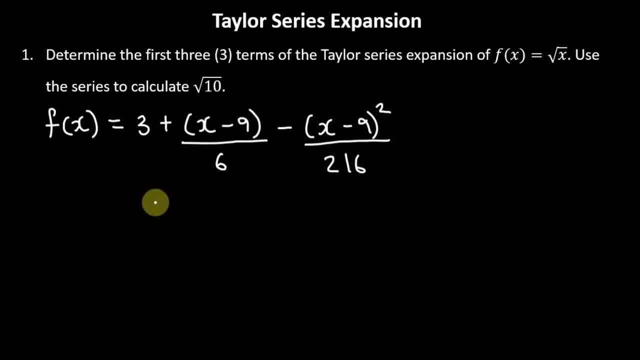 The actual square root of 10.. The reason why I say a close value and not the exact value is because we only wrote out the first three terms. The more terms you have, the more accurate your answer will be, But we should get a very, very close value. 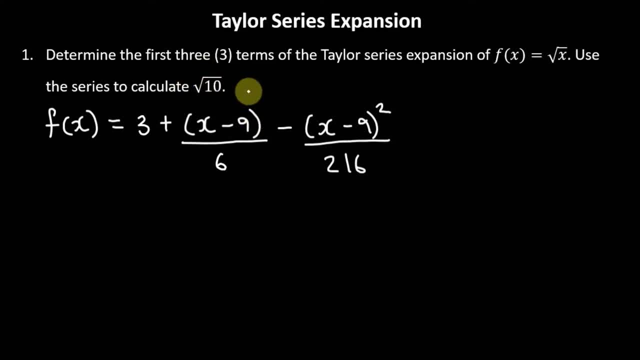 But before we use the series guys to calculate the square root of 10, let us first use our calculator to find out what is the actual value for the square root of 10.. Now, according to the calculator, the square root of 10.. 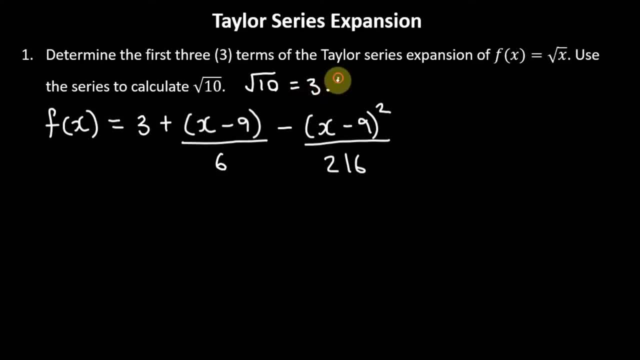 The square root of 10 is equal to three point one, six, two, two, seven, seven, six, six. So that's a value that the calculator gives us, And we're saying that we won't get that exact value, but we should be getting something very, very close. 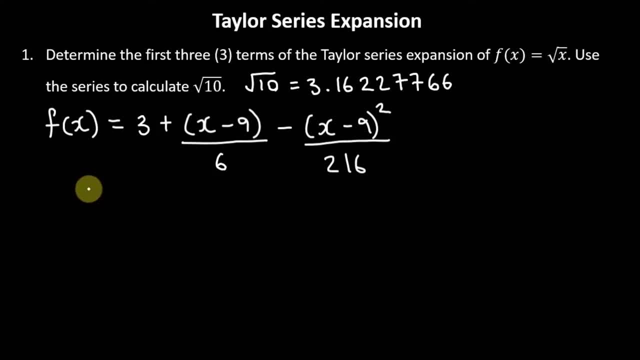 All right. So let us go ahead and see if the Taylor series expansion actually works. So here we have f of 10, or x value would be 10 here, Because this series is an expansion of the function, f of x is equal to the square root of x. 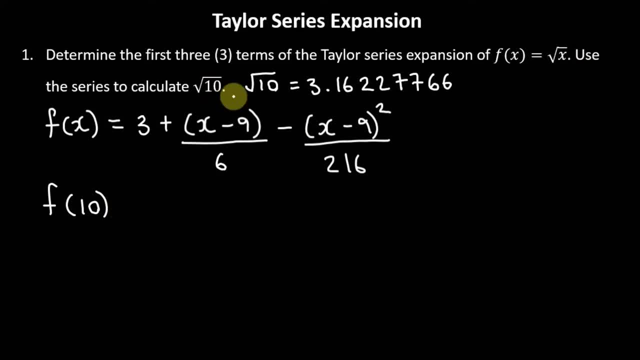 All right, So we can use it to find square root. And remember, we use a value bearing in mind that we want to find the square root of 10.. So our a value was nine, which is a perfect square, and the closest perfect square to 10.. 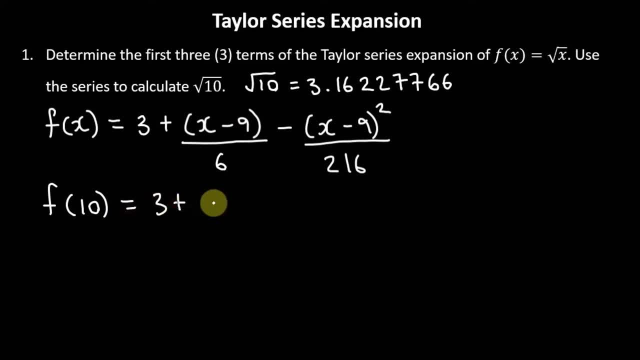 So we have: f of 10 is equal to three, So wherever we have x, we'll replace the x with 10.. We'll have 10 minus nine, So we have f of 10 over six. we have a minus sign here. we'll have 10 minus nine squared over two: 60, and let's simplify this and see what we'll get. 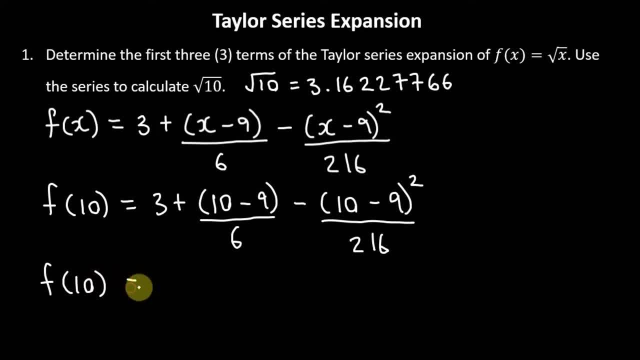 So we have: f of 10 is equal to three plus 10 minus nine is of course one, So that's one over six. So we have: f of 10 is equal to three minus 10 minus nine- Again, that's one. 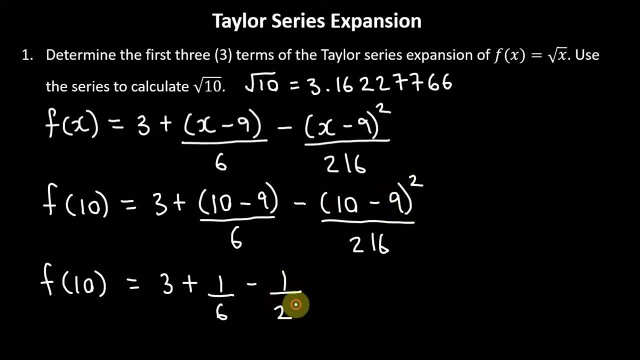 One squared is one. We have one over two, 16, and let's see what this give us guys. Again, you can work this out. You can convert these to decimals, But, of course, if you have a good calculator, you can plug in these values and the calculator will do the work for you. 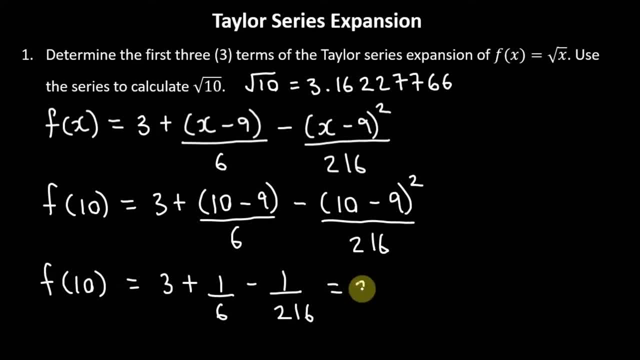 Now, when I plug this into my calculator, guys, I got three point one, six, two, Zero, three, seven, which is pretty close to the actual values, Right? So I actually got the first three decimal places, All right, But of course, as we mentioned before, it won't be as accurate because we just found the first three terms. 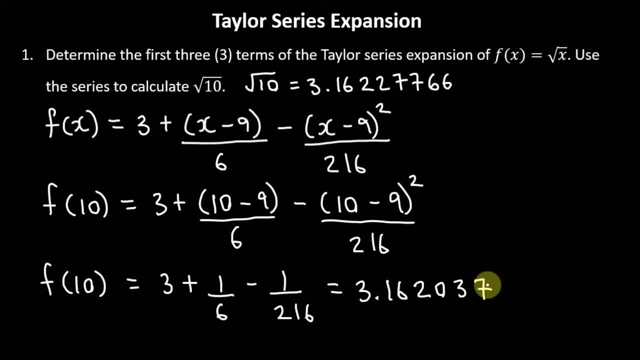 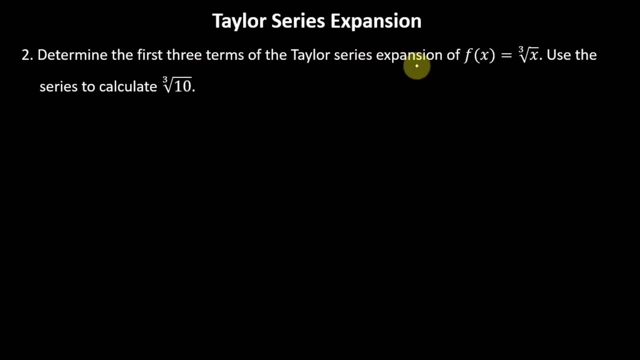 All right. So the more terms you find, the more accurate the answer will be. So, therefore, the Taylor series expansion, as we can see here, is pretty cool. All right, So let us look at question two Now. question two asks us to determine the first three terms of the Taylor series. expansion of f of x is equal to the cube root of x. 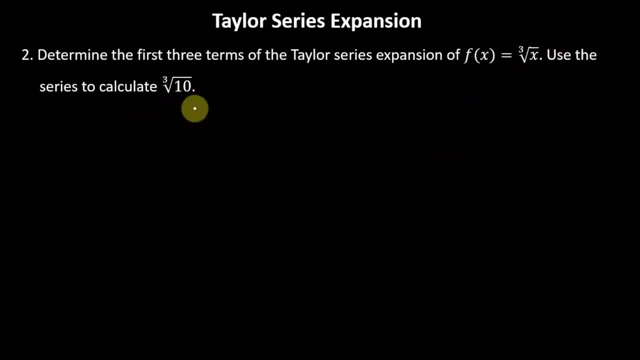 And I want to use this, the series, to calculate the cube root of 10.. All right, So the first one we looked at was, of course, the square root. It was a function. f of x is equal to the square root of x. 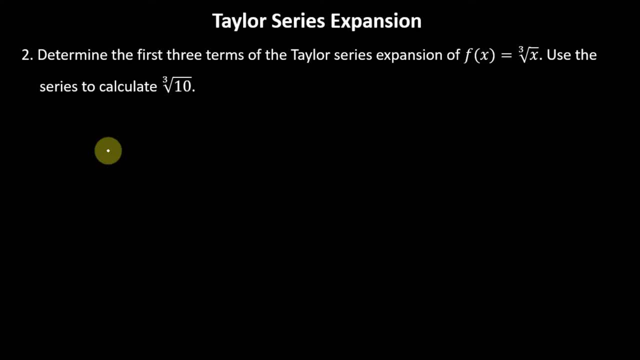 Now we want to find Taylor series. expansion of the function f of x is equal to to the cube root of x, and we have to bear in mind guys that want to use a series to calculate the cube root of 10. and again, we want to start off by looking at our formula for the Taylor series. 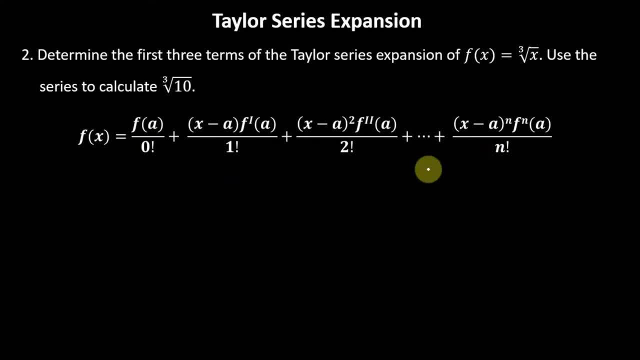 expansion. here's our formula. by now you'll be familiar with it. and again, guys, we're going to need our a value. bear in mind that the a value is dependent on the function that we want to write expansion for, as well as what we want to use it to calculate. we want to use it to calculate the. 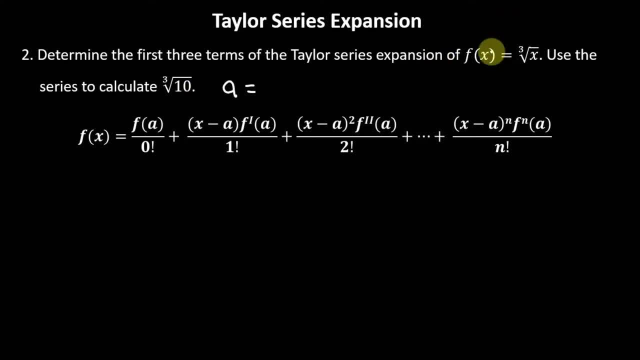 cube root of 10. all right, and of course the function is f of x is equal to the cube root of x. so, based on what we did, guys in question one, what I want you guys to do for me is to let me know in the comment section what do you think the a value will be, so you can write it like: a is equal to. 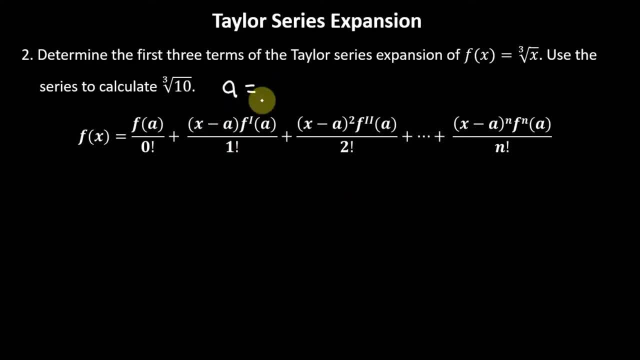 whatever you think that number will be and let's see how many of you guys will answer it- actually get it correct. you can pause the video if you need more time to think about it before i actually give you the a value. all right, now that you guys are back, i hope many of you guys got it correct, so our a value for this. 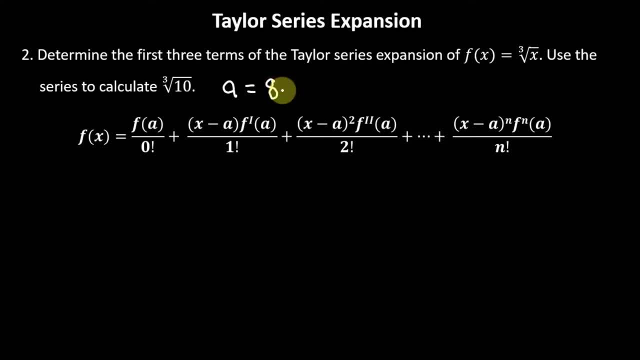 particular problem will be 8. all right, and again, the reason: 8- 8 is the closest value to 10- that when we find the cube root of this number, we'll get a whole number as the result. bear in mind that when we find a cube root of 10, of course we'll get a decimal value. now let's get right down to. 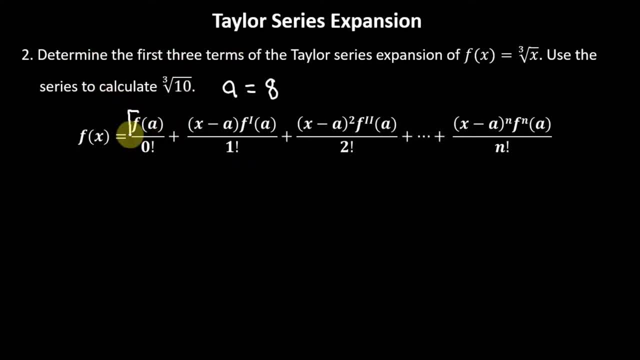 business. this also asks us for the first three terms. so we know that we are going to need our f of a first differential of f of a and also the second differential of f of a. so we're going to go ahead and find our f of a. 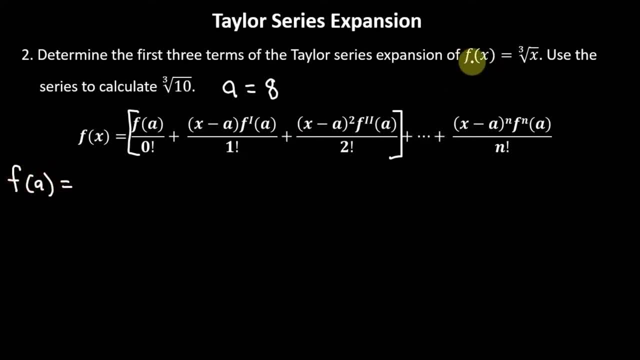 and And, of course, guys, being that f of x is equal to the cube root of x, then f of a will be equal to- there you go, the cube root of a. Now our a value is 8, so therefore, f of a will be equal to the cube root of 8.. 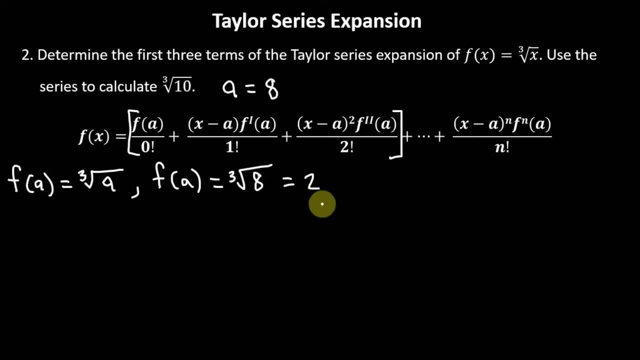 And of course the cube root of 8 is 2, which means our f of a value again. so therefore f of a will be equal to 2.. Now we're going to need to find the first differential of a. 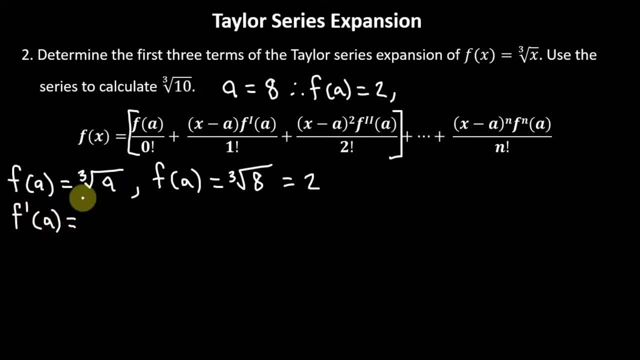 So the first differential of a. And again, guys, we're going to differentiate our f of a function And we're going to rewrite the f of a function, just like question 1.. So The cube root of a is the same thing as a raised to the power of 1. third, 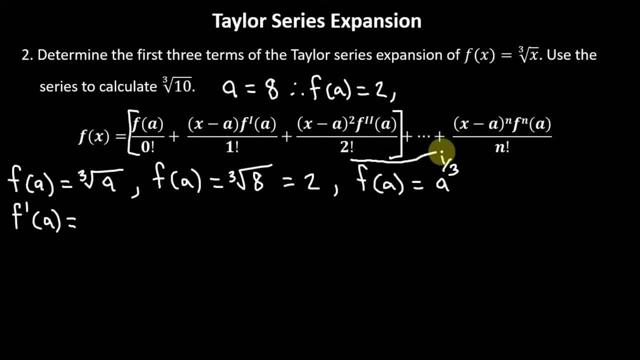 And again, guys, the reason why I do this. this is probably easier to look at when we're thinking of differentiation than the actual cube root sign right here. So in differentiating this function, we'll multiply by the power, So we have 1 third times a. 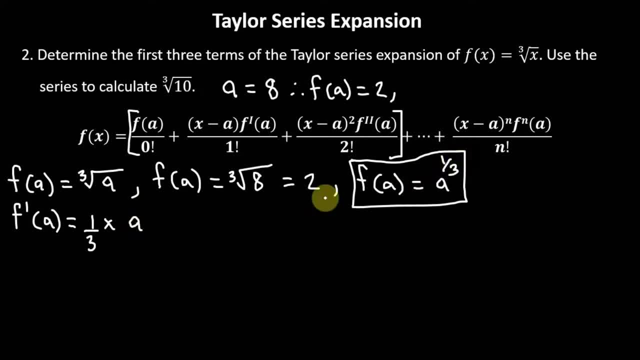 And of course we'll minus 1 from the power, 1 third minus 1.. We'll of course Give us negative 2 thirds. All right, And of course again, guys, we can clean this up. So the first differential of f of a is equal to 1 times a raised to the power of negative 2 over 3.. 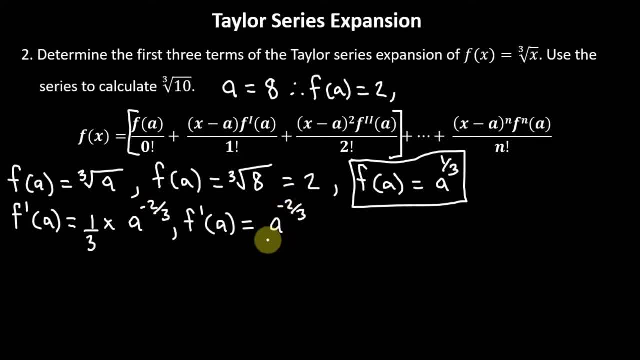 That is of course a to the power of negative 2 over 3.. And we'll have the 3 in the denominator here And we can go a step further. By now. you know you can apply the laws of indices. 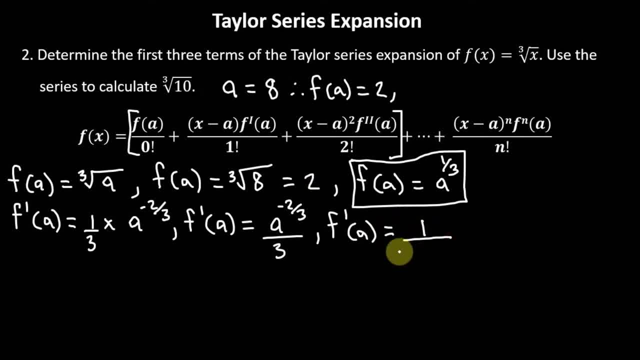 So we'll have 1 over 3.. And in bracket, here we're going to have the cube root of a in bracket squared And recall guys that our a value is 8. So we can plug that value in here. 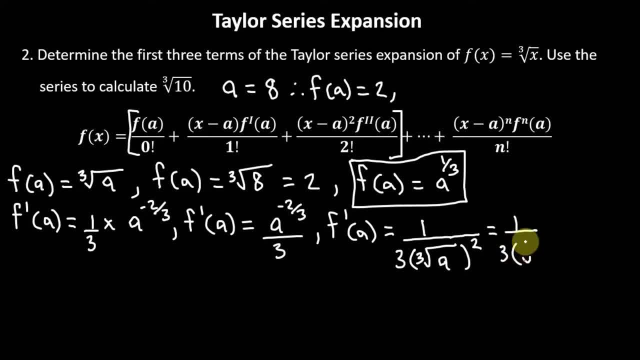 So we'll have 3 in bracket, the cube root of 8. Squared. And what will this give us? 1 over. Let's see: The cube root of 8 is of course, 2.. 2 squared is 4.. 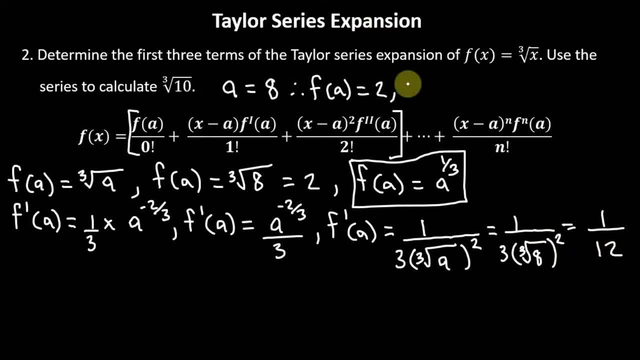 And, of course, 3 times 4 is 12.. So, therefore, the first differential of f of a we can say is equal to 1 over 12.. And now, guys, we need to find the second differential of f of a. 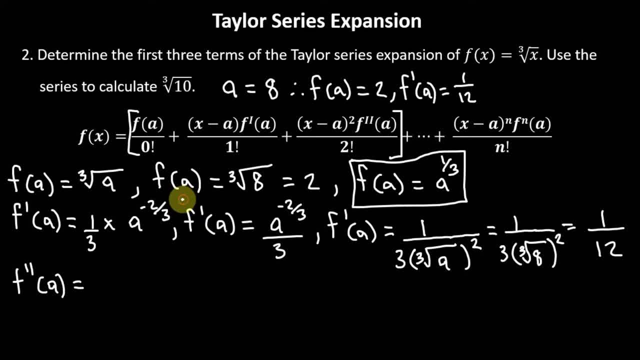 All right, And again We can use this function. here We're going to need the first differential of f of a function And we're going to use this one Now. again, we'll multiply by the power guys, So we're going to have negative 2 thirds times. 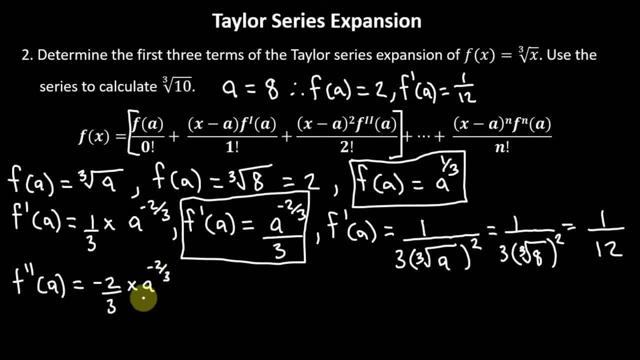 We have a raised to the power of negative 2 thirds here over 3.. And recall that will minus 1 from the power. So negative 2 over 3 minus 1. That will give us negative 5. 5 over 3.. 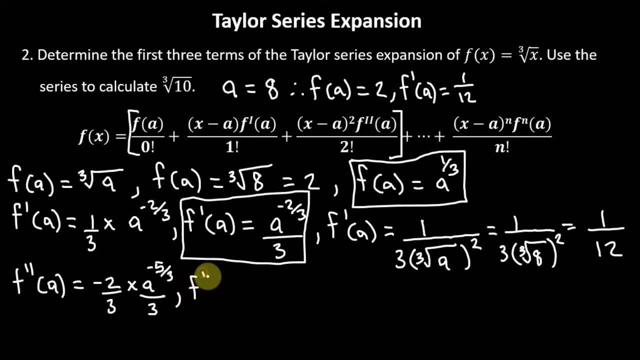 All right, And again, guys, we can clean this up a little bit. So we have: the second differential of f of a is equal to, And, of course, negative 2 times a, raised to the power of negative 5 over 3.. 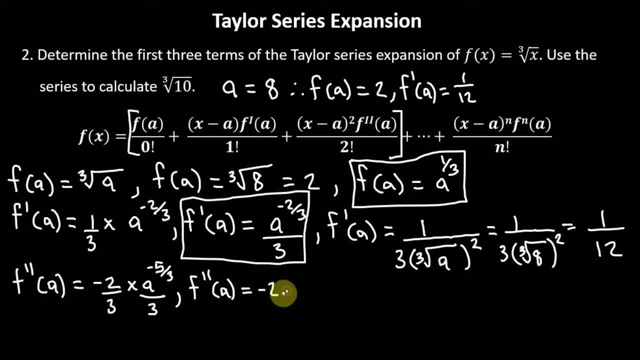 Will, of course, give us negative 2a a raised to the power of negative 5 over 3.. All over 3 times 3 is, of course, 9.. And where do we go from here? Of course, guys, we can clean this up a bit more using the law of indices. 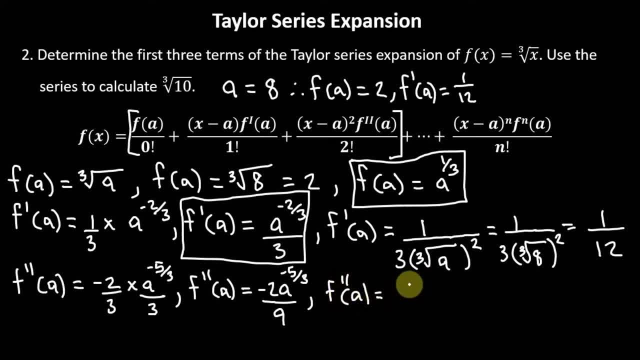 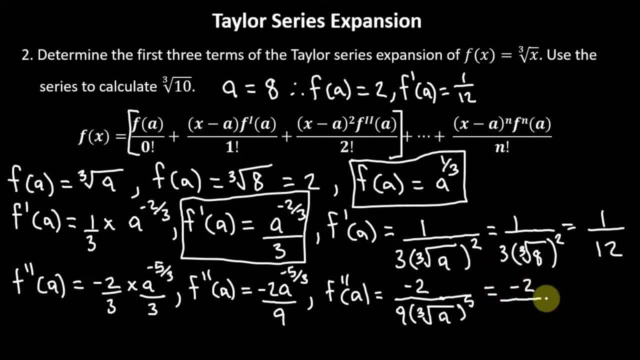 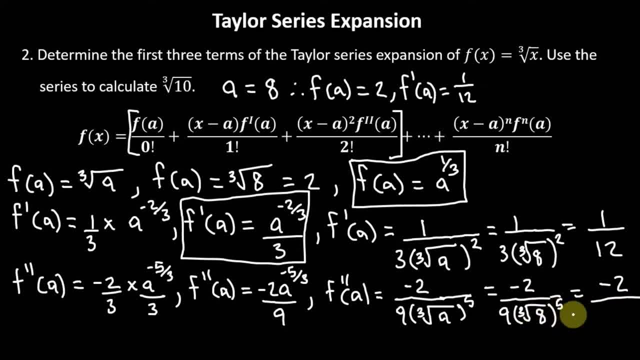 The cube root of 8 is of course 2.. 2 raised to the power of 5 is 32.. And of course 9 times 32 will give us 200. And of course we can reduce this guys. 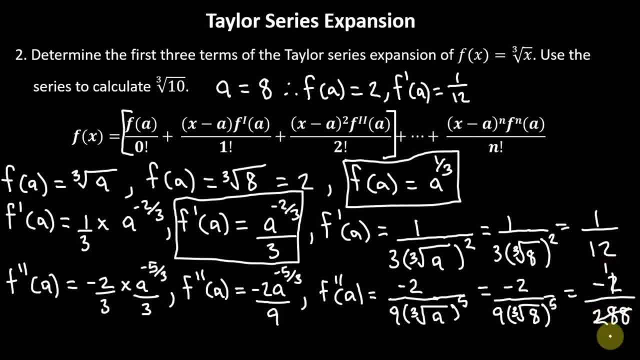 So 2 into itself, 1.. 2 into 288 will give us 144.. So therefore we can say the second differential of f of a is equal to negative 1 over 144.. And again, guys, this is majority of the work done here. 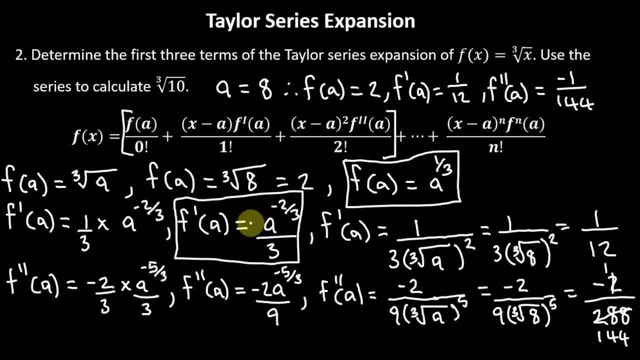 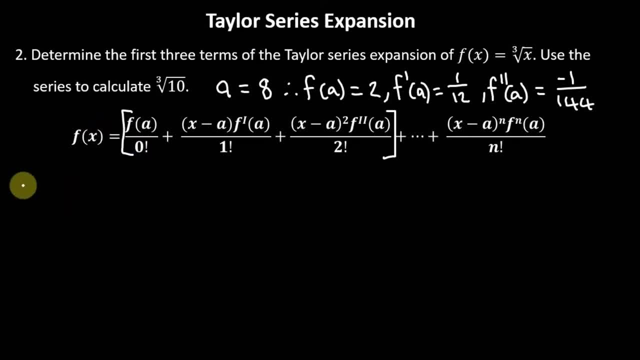 So we're going to clear this space again And then write out the first three terms. Now, to write out the first three terms, guys, we're going to use the Taylor series expansion formula to guide us. So we're going to have: f of x is equal to the value that we got, for f of a was, of course, 2.. 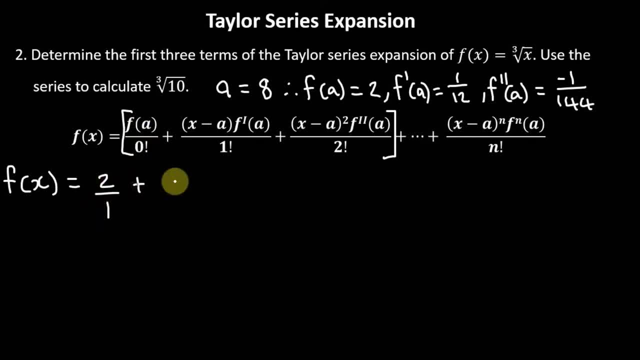 We'll have this over 0 factorial, which is 1.. Plus we're going to multiply this bracket here by the value that we got for the first differential of f of a, which was 1 over 2.. So 1 over 12 times the bracket here: x minus a. 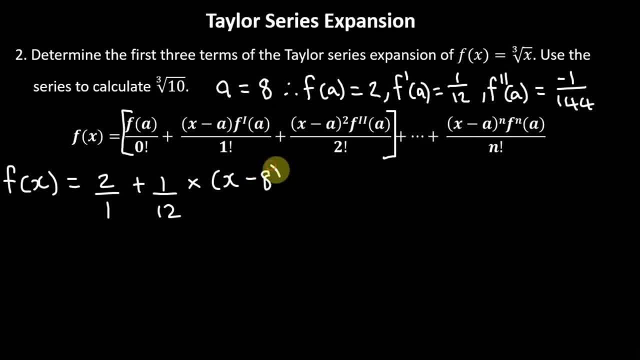 And of course, the value for a is 8 over 1 factorial, which is 1.. Plus, we're going to multiply this bracket here: x minus a, all squared by the value that we got for the second differential of f of a, which was negative: 1 over 144.. 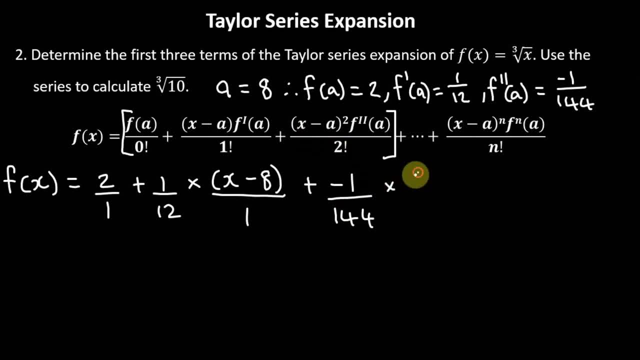 And we'll multiply this by the bracket here, So we'll have x minus and, of course, guys, the value for a is of course 8.. And raise this to the second power And we'll put this over 2, factorial, which is 2.. 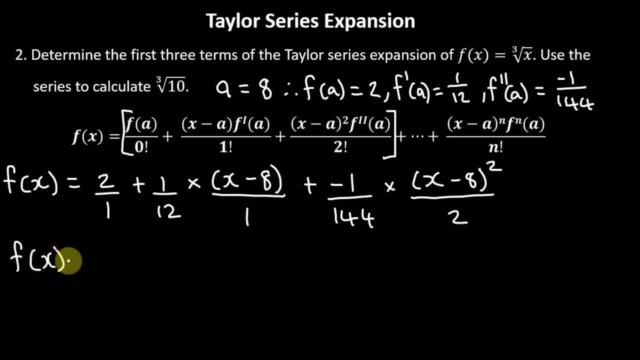 And we can always clean this up a little bit, So we'll have: f of x is equal to 2, divided by 1 is 2.. Plus 1 times x minus 8 in bracket will remain x minus 8 in bracket. 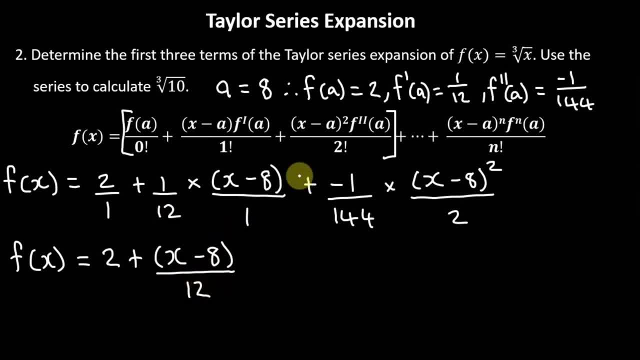 12 times 1 is 12., And whenever we have a positive and a negative sign beside each other like this, they're equivalent to a minus sign. So we'll have minus and we'll have 1 times the bracket here. 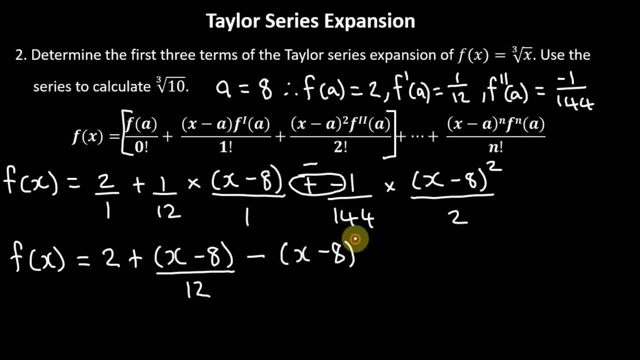 Of course it will remain x minus 8 in bracket. squared all over 144 times 2 is of course 288.. This is pretty much the first three terms of the Taylor series. expansion of the function f of x is equal to the cube root of f of x. 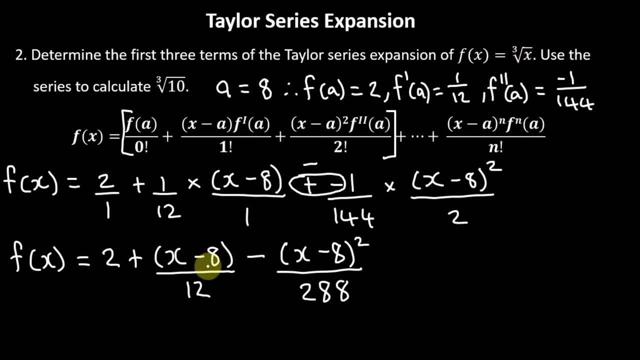 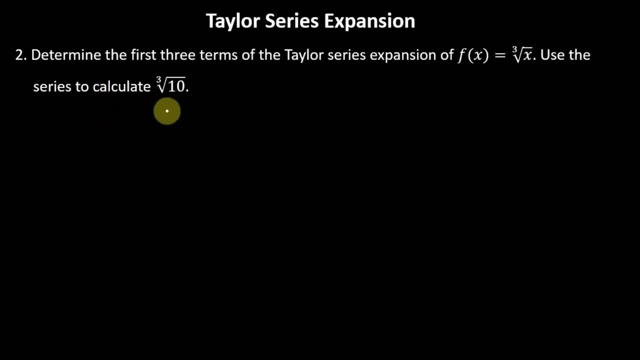 So we'll have x minus 8 in bracket, squared all over 144 times 2 is of course, 288.. Now we want to use the series to calculate the cube root of 10.. Now, as we mentioned before, guys, we want to use the series to calculate the cube root of 10.. 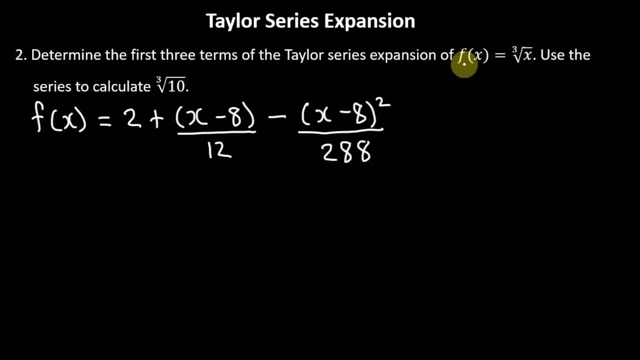 Now recall the series. So this is the Taylor series. expansion for the function f of x is equal to the cube root of x, bearing in mind that we wanted to use the series to calculate the cube root of 10.. And we chose our a value, as we would have seen before, bearing that in mind. 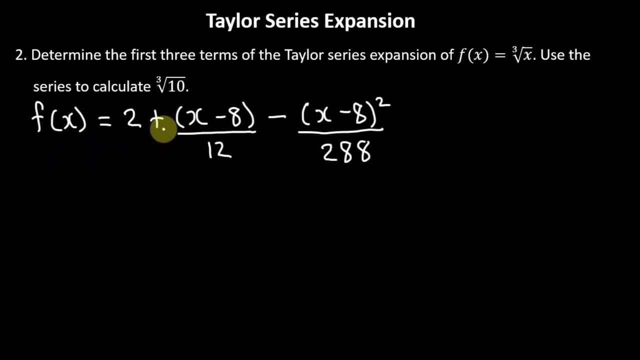 So, um, This is a function. f of x is equal to 2 plus x minus 8, in bracket over 12 minus x minus 8, all squared over 288.. So, um, We're going to use this now to find the cube root of 10.. 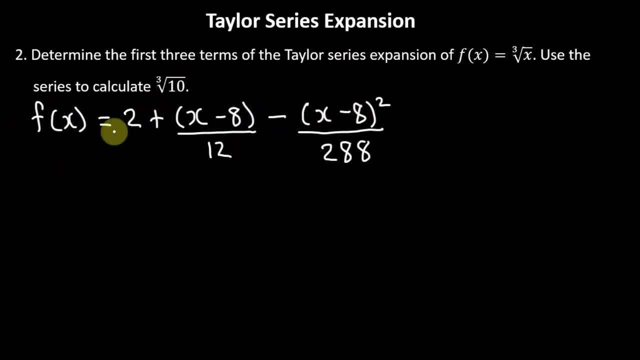 And that is pretty much what this Taylor series expansion was for. So we wrote just 3.. It was 3.. And remember guys, we can have an infinite amount of terms, But we just Wrote out the first 3.. 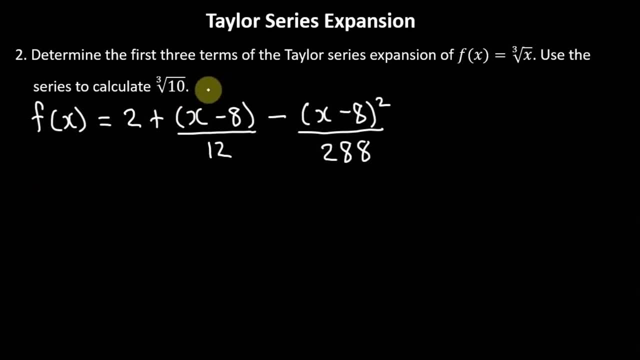 So therefore, again, this answer will not be the exact value for the cube root of 10.. So, bearing that in mind, let us go to our calculator and first find out what is the exact value for the cube root of 10.. 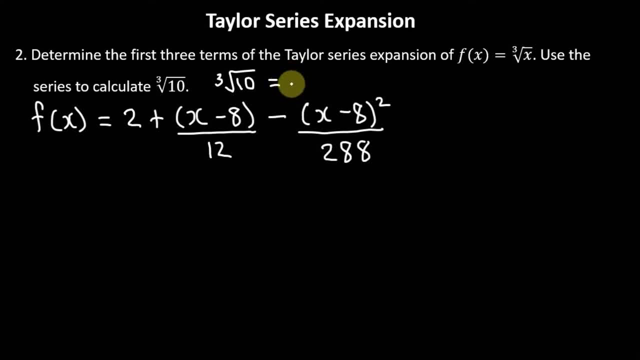 Now the value that I got from my calculator was that the cube root of 10 was 2.15443469.. So that's the value that I got, guys. So let's see how close the Taylor series expansion result will be. 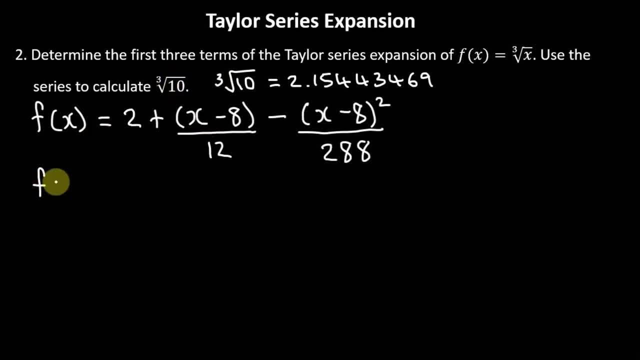 So, um, I want to find this cube root of 10.. So I'm going to plug 10 into the series here. So we have: f of 10 is equal to 2 plus Wherever we have x, we replace the x with 10.. 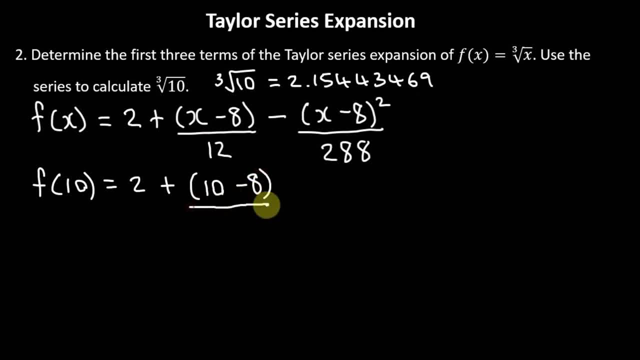 10 minus 8 over 12 minus 10 minus 8.. 8 raised to the power of 2 over 288.. Of course guys again Can clean this up a little bit. So we'll have 2 plus. 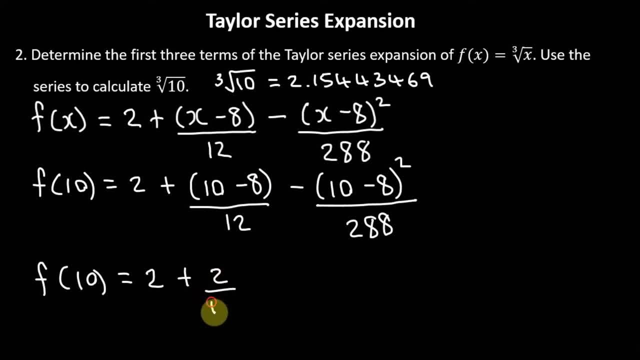 10 minus 8 is of course 2.. So we have 2 over 12.. Minus 10 minus 8 is of course 2.. 2 squared is 4.. So we'll have 4 over 288 here. 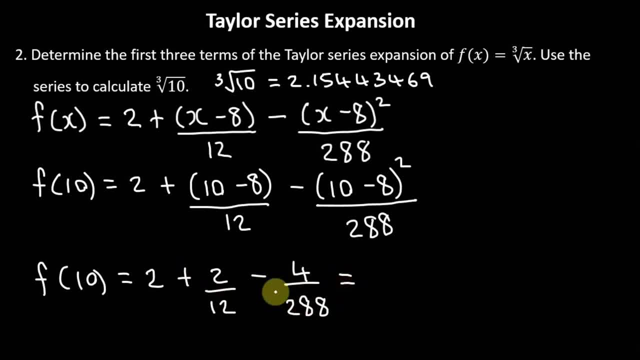 And we can plug this in Into our calculator and get a value. You can simplify it if you wish to, But of course you can use a calculator to do the work for you And we can see how close our result will be toward the actual value of the cube root of 10.. 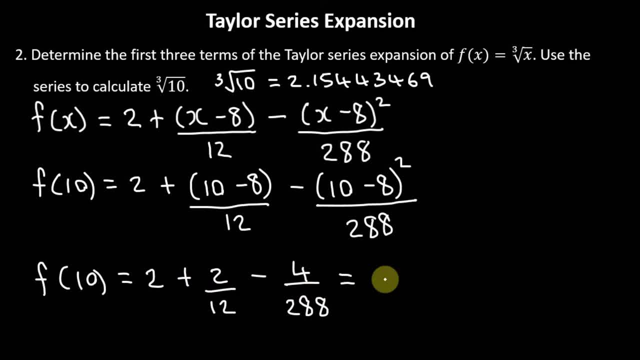 And the value that I get, guys. when I plug this into my calculator, I got 2.1527.. Which, again, is pretty close to the actual value. So, as you can see here, guys, The Taylor series is pretty cool. 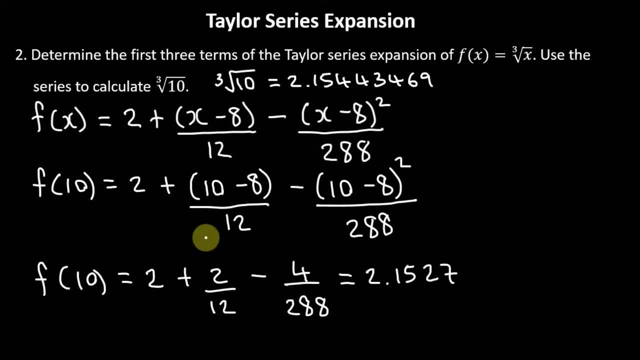 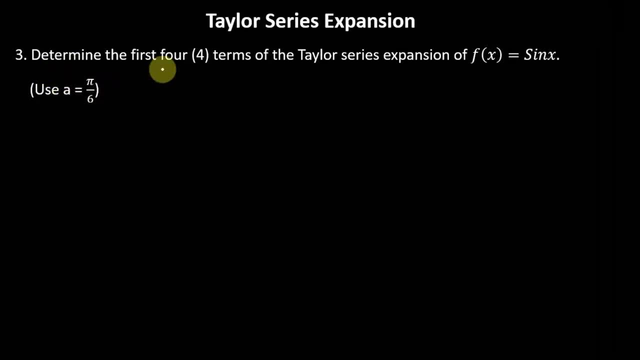 And it works pretty well. Alright, Now to look at our final example. guys, We are going to look at a trig function. Now we're looking at question 3.. Determine the first 4 terms of the Taylor series. expansion of f of x is equal to sine of x. 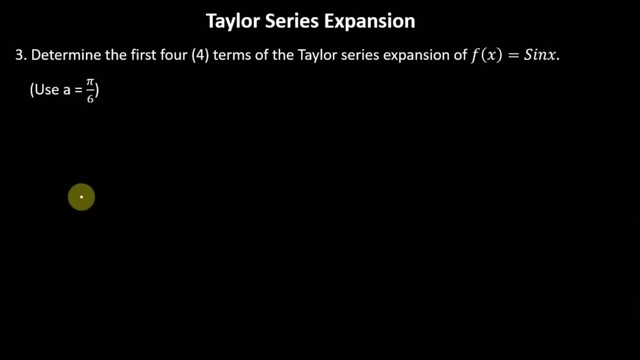 And here they gave us the, a value which is pi over 6.. And, as always, guys, we always want to have our formula here to guide us throughout the entire process. Now, here we have our formula, guys, And, unlike the previous examples, they want us to find the first 4 terms. 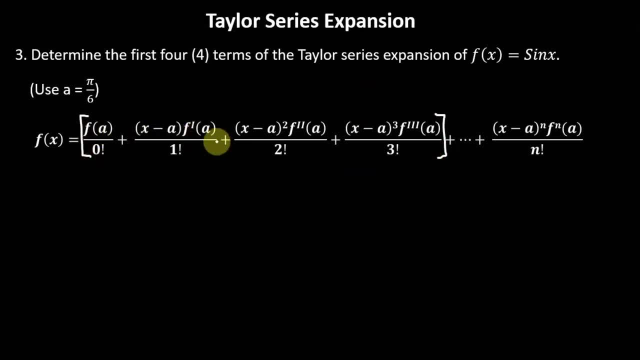 Which means we are going to need to find f of a, the first differential of f of a, the second differential of f of a and also the third differential of f of a. So the concept remains the same. Bear in mind also, guys, that a here pi over 6, is the same thing as 30 degrees. 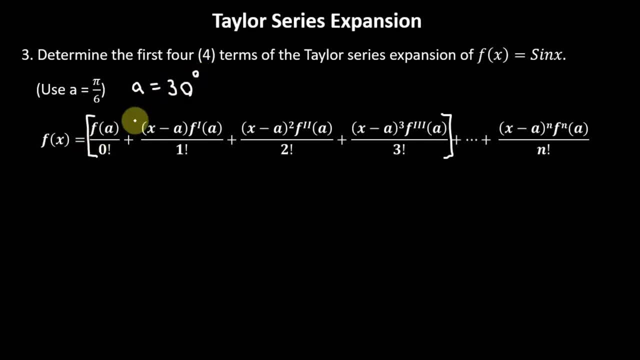 I think you guys probably know how to convert from radians To degrees. alright, We are going to use the formula to guide us, of course. So we are going to need to find our f of a And, of course, if f of x is equal to sine of x, then f of a will be equal to sine of a. 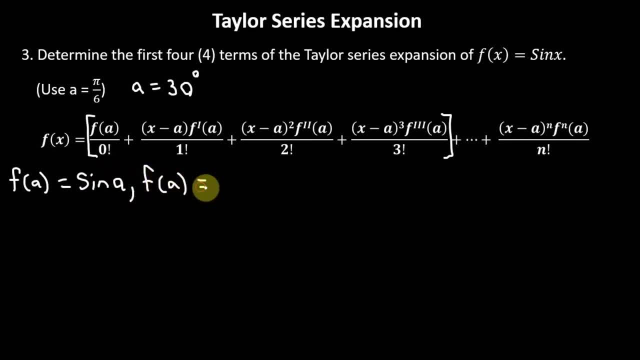 So, therefore, f of a will be equal to sine of 30 degrees, Which you can find in your calculator quite easily, And of course, sine 30 is a half. Next step is to find the first differential of f of a. 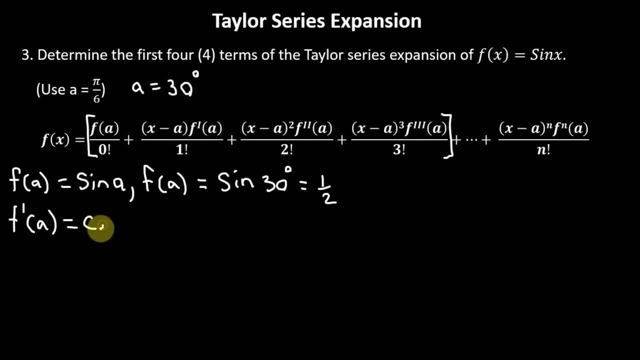 Of course, when we differentiate sine a, we'll get cos a. So therefore the first differential of f of a will be equal to cos of 30 degrees, Which is of course root 3 over 2.. Next we'll find the second differential of f of a. 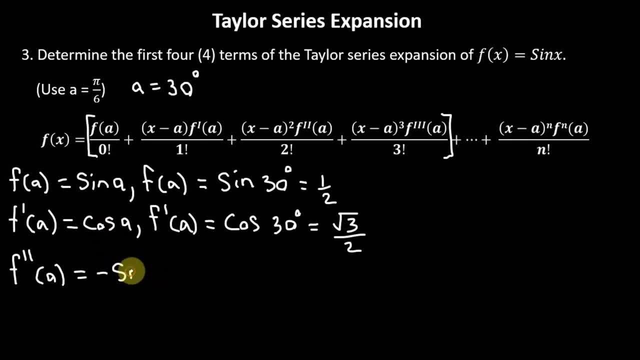 And when we differentiate sine of a we'll get cos of 30 degrees And of course sine of a will be equal to cosine of 30 degrees. cos A will end up with minus sine A, which means the second differential of F. 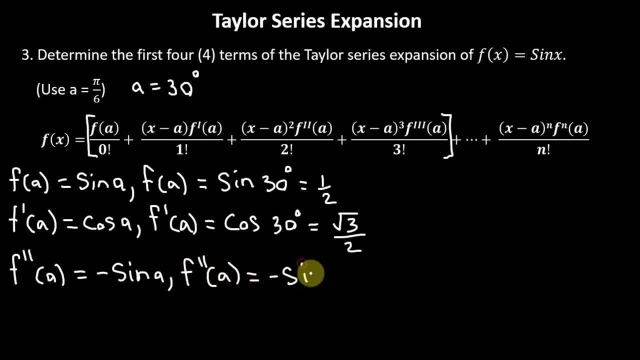 of A will be equal to minus sine of 30 degrees, which is equal to negative 1 half. and finally, guys, we'll find the third differential of F of A and, of course, when we differentiate minus sine A will end up with minus cos A, which means the third differential F of A will be equal to minus cos of 30 degrees. 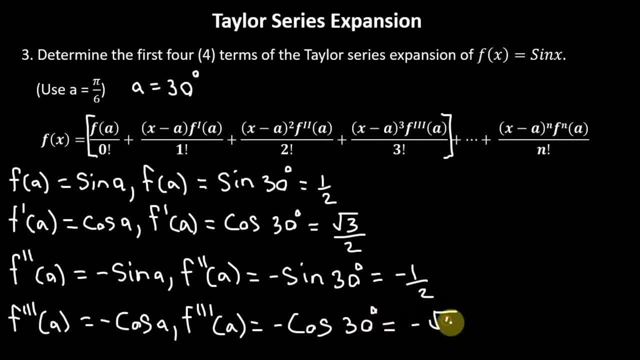 which is minus root, 3 over 2, and these are values, guys, that we need in order to write out the first four terms and we can have them here as well and some going to have to erase down here. so F of A, it's a half. 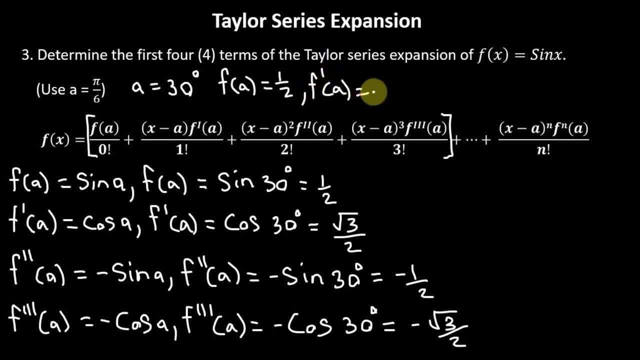 F of A. differential of f of a is root 3 over 2.. Second differential of f of a is minus a half. And, of course, the third differential of f of a is minus root 3 over 2.. Now we're going to. 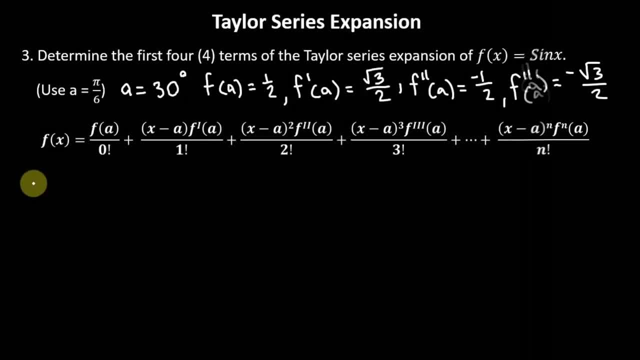 erase this space and then write out the first four terms. Now our final step is just to write out our first four terms, which we can do with the aid of our formula here. So we'll have: f of x is equal to, or f of a value which was a half. So we'll have half divided by. 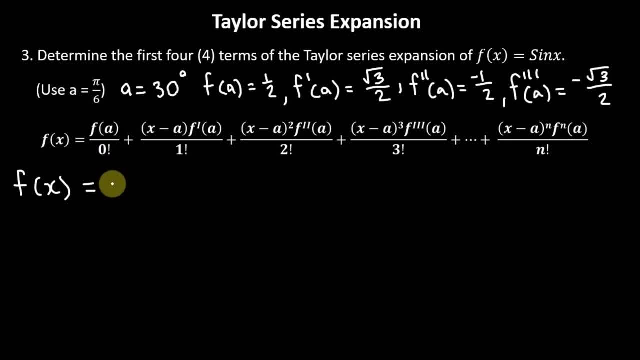 0 factorial, which is 1.. A half divided by 1 is still a half Plus. we'll multiply this bracket here x minus a in bracket by the value that we got for the first differential of f of a, which was 1. Plus root 3 over 2.. So we'll have root 3 over 2 times the bracket here x minus a, And we'll 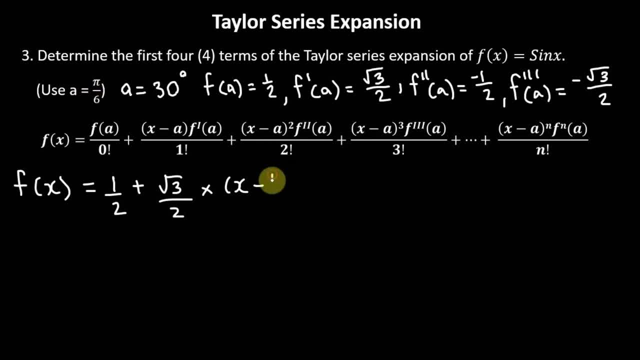 just replace a with the a value that they gave us: Pi over 6.. Of course, this is the same thing as 30 degrees, but we'll just use back the value that they gave us. We'll put it back in radian form And we'll put this over 1 factorial, which is 1.. 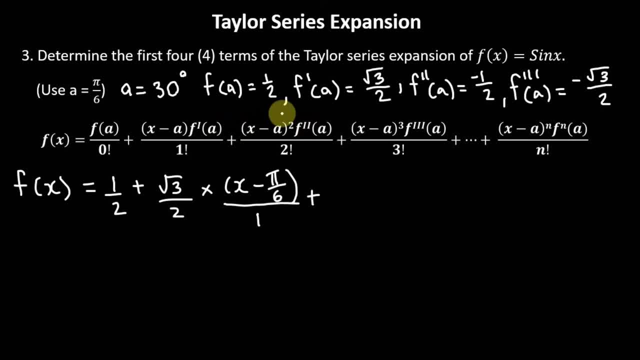 Plus we'll multiply this bracket here, x minus a in bracket, all square by the value that we got for the second differential f of a, which was 1 over 2,, 1 minus half, So minus half Times x, minus again the value for a as pi over 6.. And we'll square the bracket. 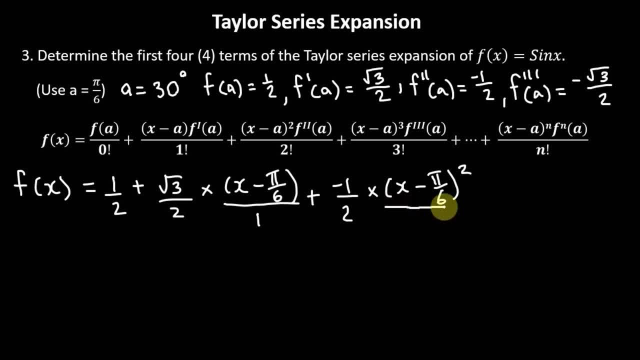 just the same And we'll put this over 2 factorial, which is 2. Plus 1alpha. this bracket here- x minus a- all cubed by the value that we got for the third differential of f of a, which was minus root 3 over 2. so we'll have minus root 3 over 2 times x minus a and again our a. 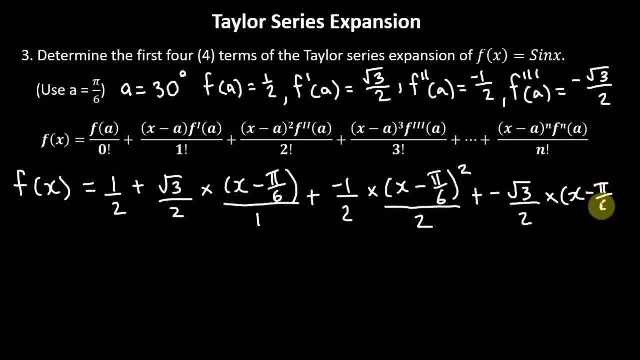 value is pi over 6, and we'll cube the bracket just the same and we'll put this over 3 factorial, which is of course 6, and of course, guys, we can clean this up a little bit, as I always like to say, so it look a whole lot more presentable. so let's keep the half here, plus, of course, we have. 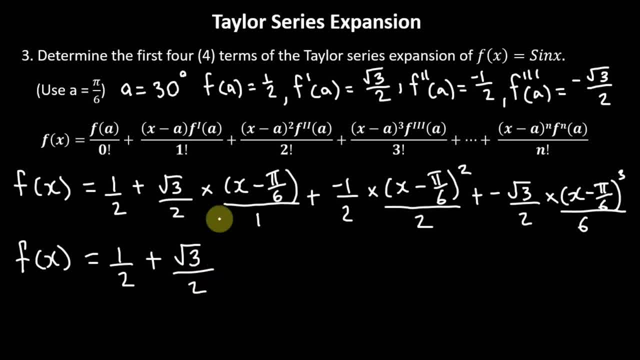 root 3 times the bracket here. so root 3 times x minus pi over 6 in bracket. and of course, once we have an addition and a minus sign here, the combination of both signs is always equivalent to a minus sign. so we'll have minus, of course. 2. 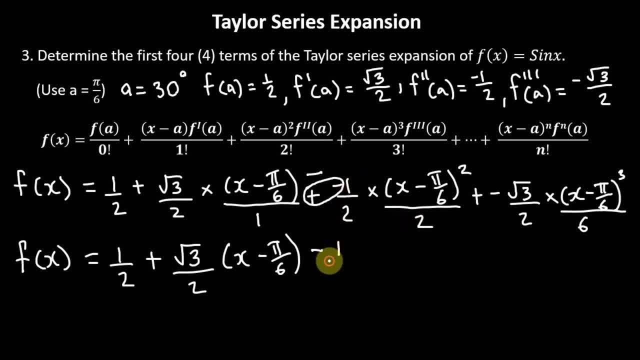 times 2 is 4, so we can have a quarter here. times this bracket here, which is x minus pi over 6 all squared, and again combination of a positive and a negative sign is always equivalent to a negative. so we'll have minus root 3 over 2 times 6 is of course 12. so root 3 over 12 times this bracket. 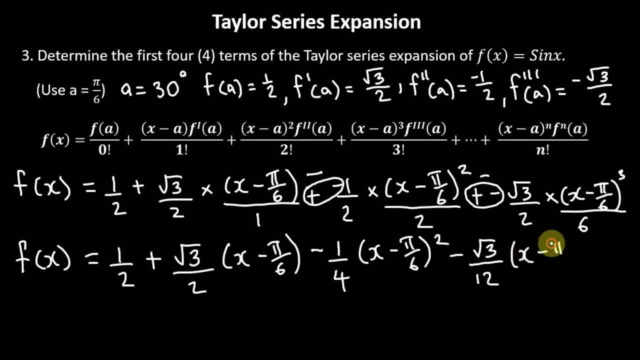 here, which is x minus pi over 6 all cubed. and that is it for this video, guys. I hope this video was beneficial to you. as I said before, this video was requested by two of our viewers and I'm sure others out there would have desired this video just the same, so I hope you guys enjoyed this video.